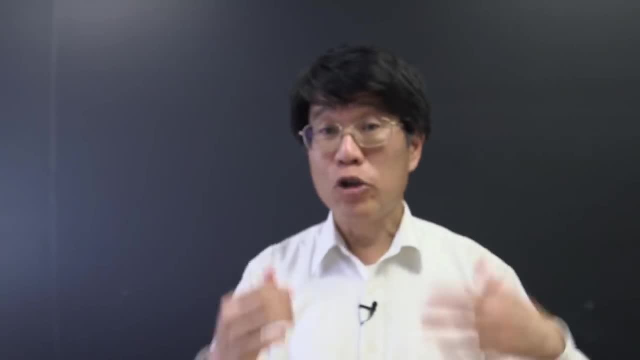 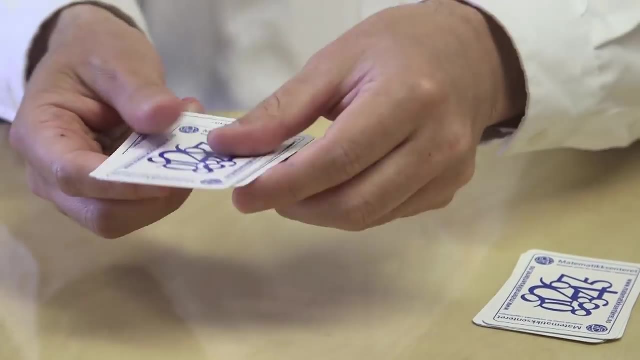 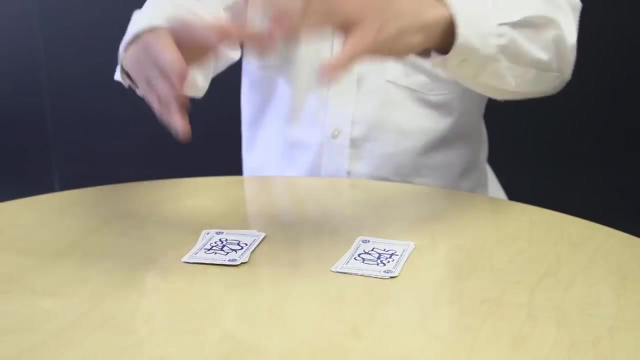 And we're going to shuffle them And you decide which one to shuffle, But the shuffling means always to take the top card and put it at the bottom. That's shuffling. Okay, That's one shuffle. And each time you tell me which one to shuffle, I'll shuffle that one. Okay, So let's shuffle a. 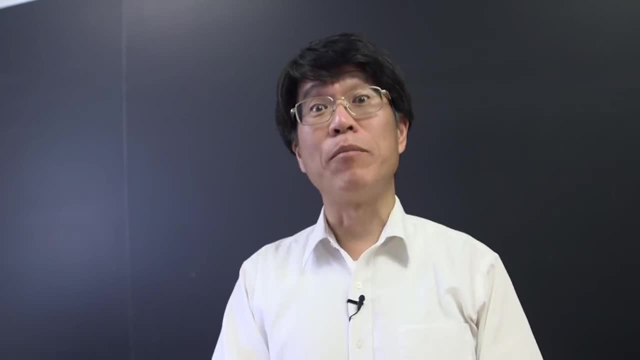 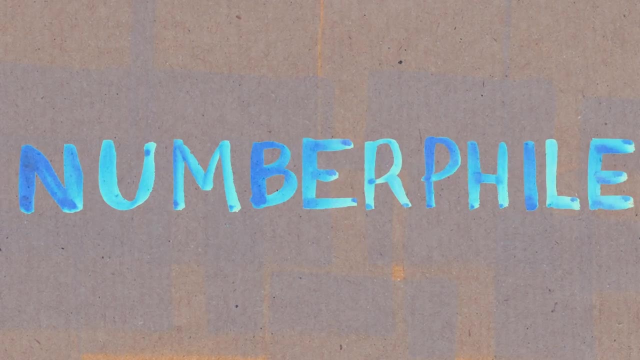 number of times. Well, what can we say? Oh, let's use the phrase number file, shall we So? number file N-U-M-B-E-R-P-H-I-L-E. So for each of these letters, you say: well, shuffle the right one, or? 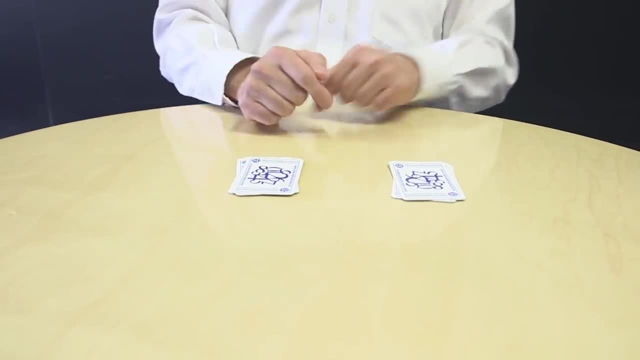 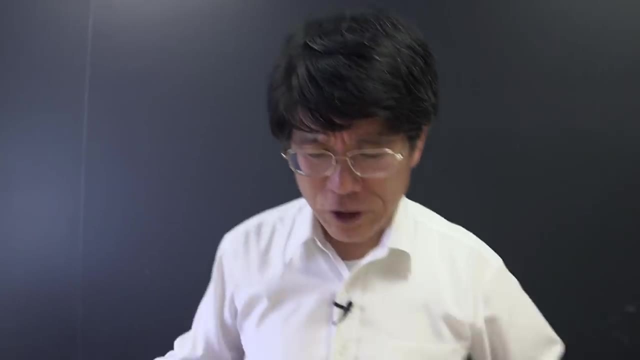 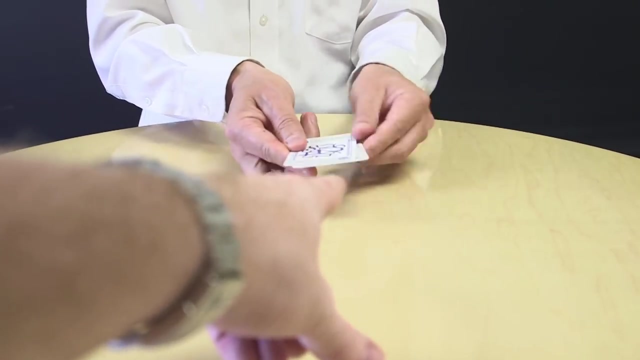 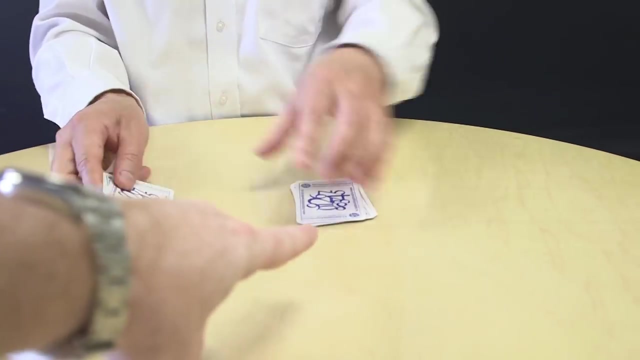 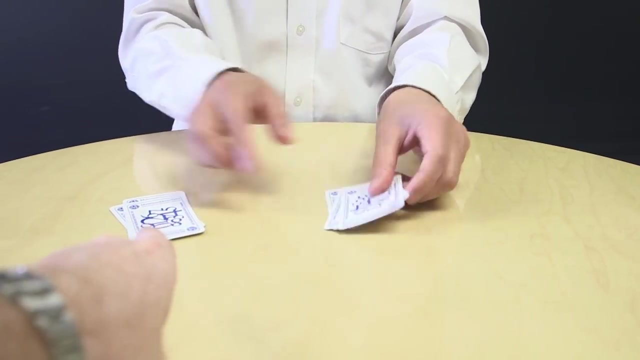 the left one, And you can say: you know, N-U-M-B-E-R-P-H and so forth, You can choose whatever you like. Okay, So, Brady, You tell me which one to shuffle then. So, left or right, Let's go N-U-M-B-E-R-P-H-I-L-E. 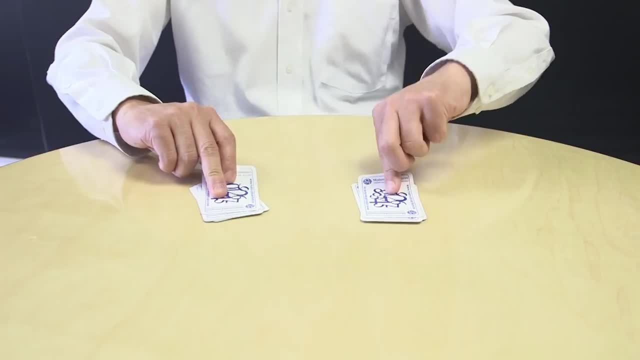 E. Okay, So those two cards emerged to the top as a result of your choice. Yeah, I didn't choose this. Yeah, So I'm going to shuffle this one. Okay, So, I'm going to shuffle this one. I'm going to set them aside. 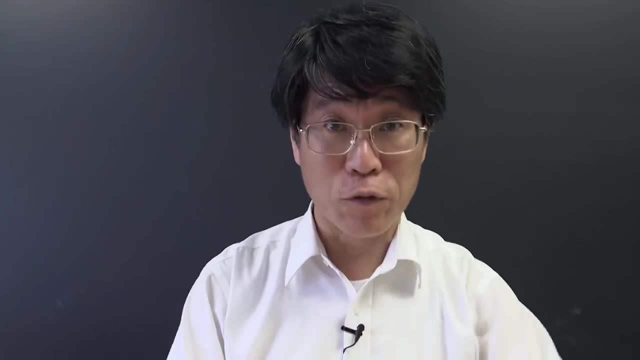 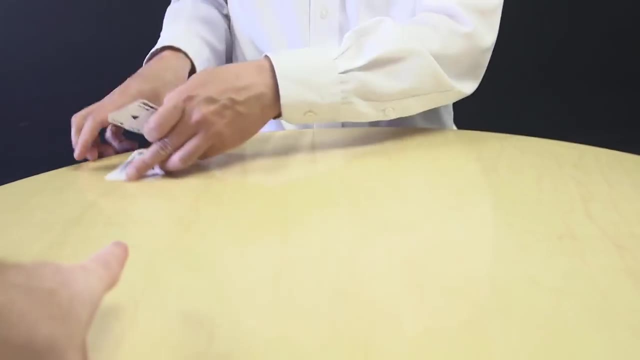 Yeah, two of them. Now we repeat number file again And for each of those letters we shuffle either of these and you choose which one to shuffle for each of those letters. So which one do you want? Let's do, let's do all of them. that one. 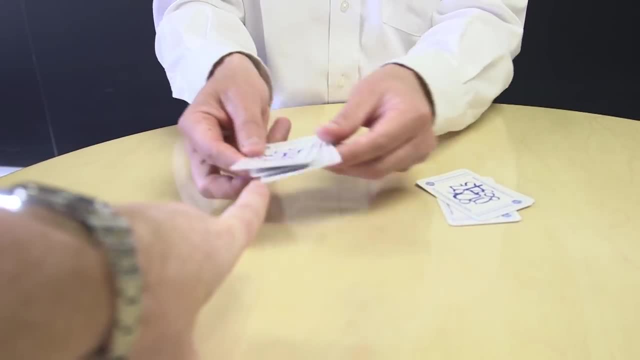 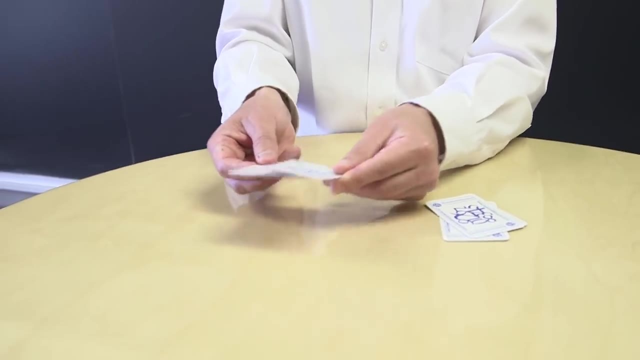 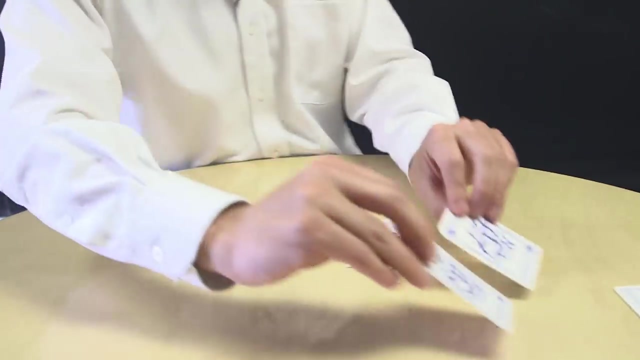 Oh, my God. So okay, M-N-U-M-B-E-R-P-H-I-L-E. I wasn't expecting this. Okay, those two cards emerged at the top. In fact, this one didn't move, but this emerged on the top. 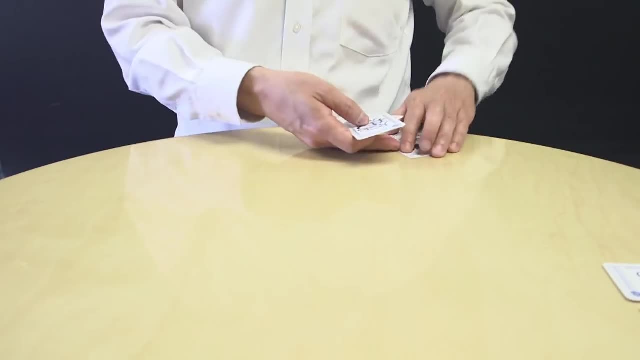 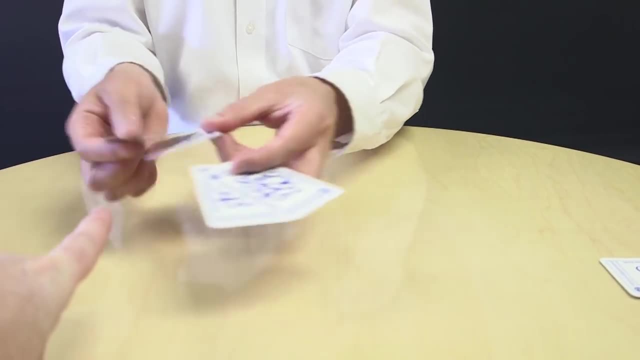 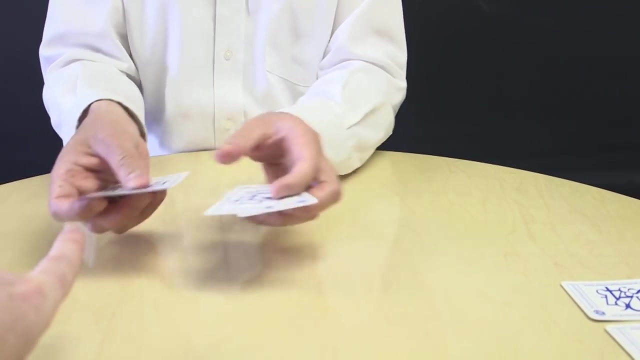 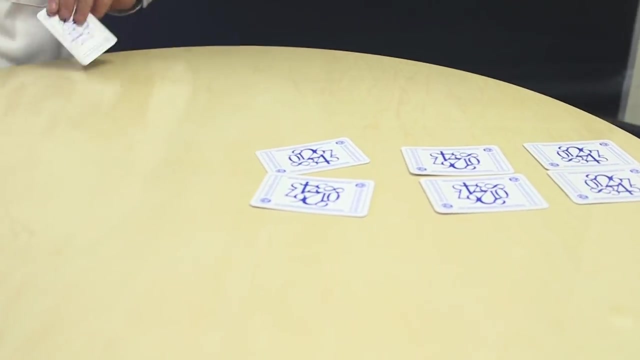 So I put these aside. Now one last time number file and you choose which one to shuffle. Okay, In whatever order: N-N-U-M-B-E-R-P-H-I-L-E. Okay, these two emerged on top and these two emerged on the top. 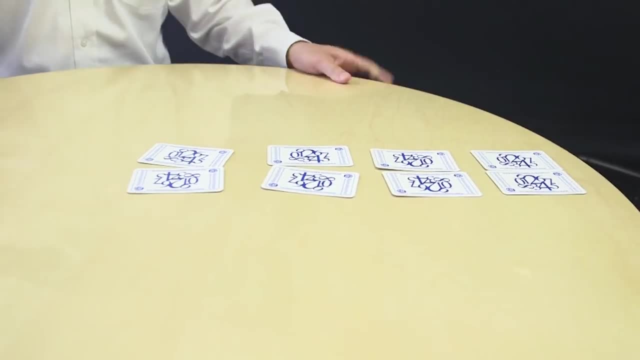 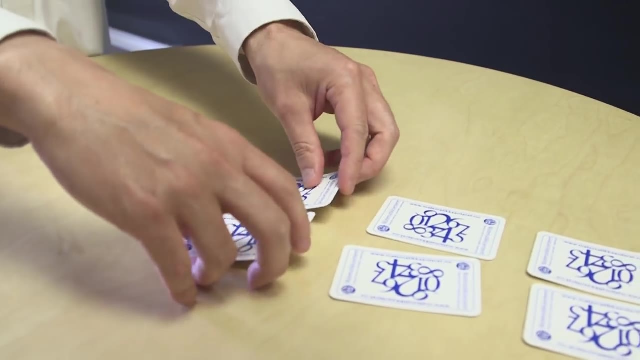 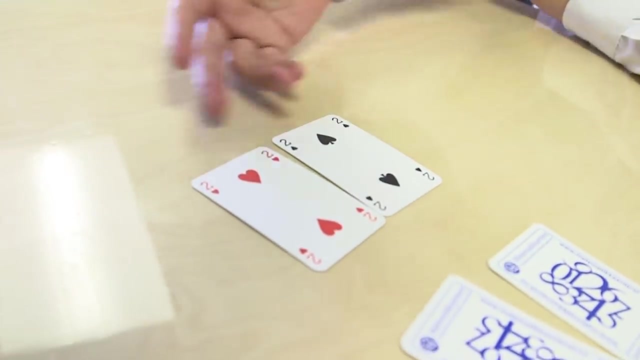 These two are left over. Okay, now, if we are really lucky- and luck doesn't come except to the deserving, because number file is such a magic phrase- these two may be the same number. You know, number file means liking numbers and these two numbers like each other, of course: two and two. 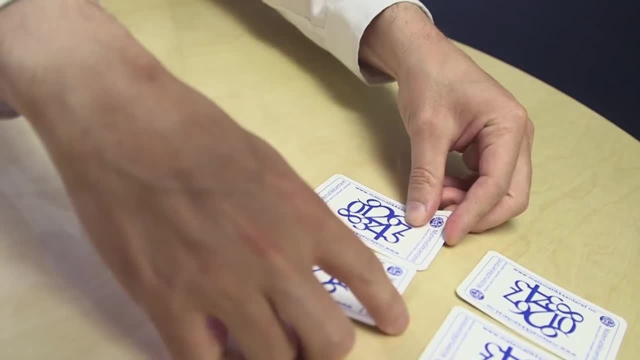 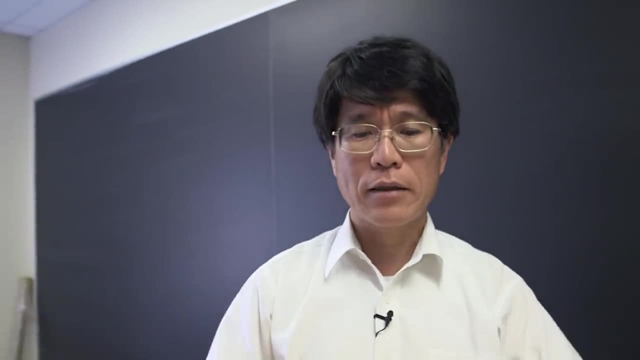 But that might have been luck. But if we really believe in the magic of number file, these two might have matched. Remember you chose which one to shuffle? Yeah, I didn't. That's surely not possible. But what's really impossible would be impossible. 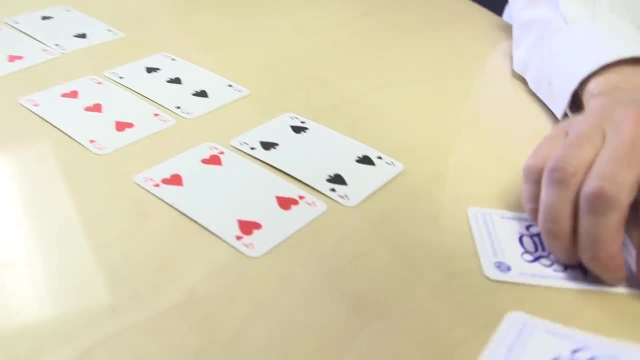 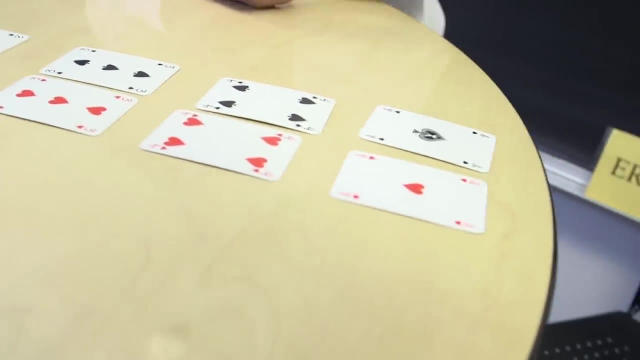 is for the next two to match And, surprise by surprise, the last two also match. So they all match pairwise. Lovely Number file. I knew it was magic. I knew it wasn't magic, So the trick that I have just shown you is a classic trick. 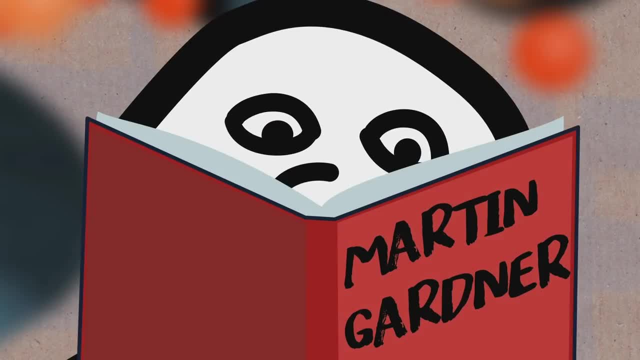 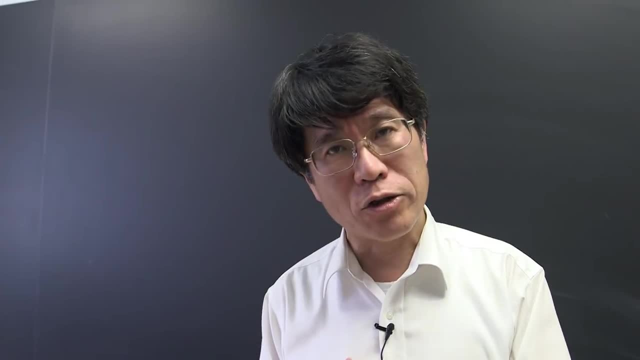 which was described for the first time, as far as I know, by the late Martin Gardner, called last cards match And I made a variation on this And the variation is a little slower than the original trick but it's also mathematically more interesting. 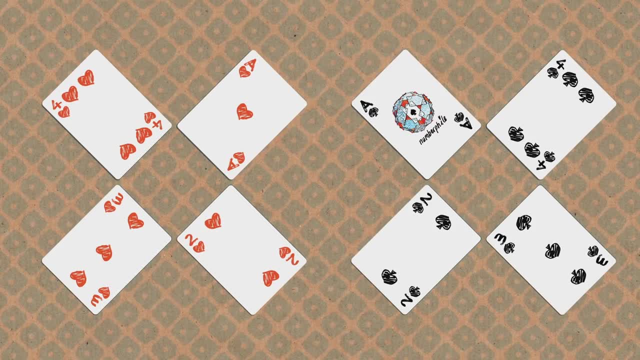 So I'd like to reveal the secret. What we had was two pairs of cards. You have one, two, three, four in one order, and one, two, three, four or, if you like, four, three, two, one in the reverse order. 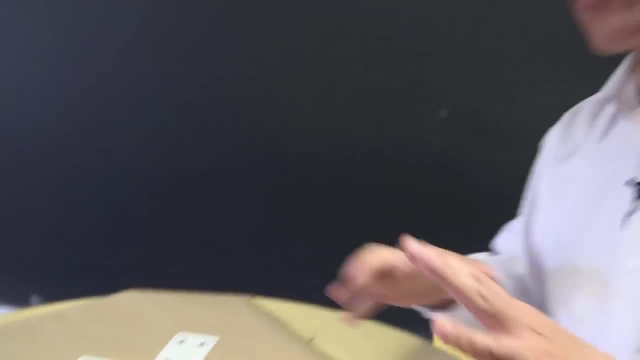 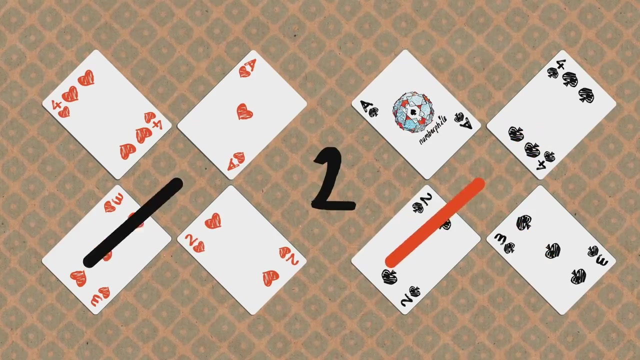 And these should be thought of as like clocks. Okay, so a clock has, you know, one, two, three, four, all the way to 12, and then it starts all over again. So you are doing modular arithmetic Here. also, if you go one, two, three, four, 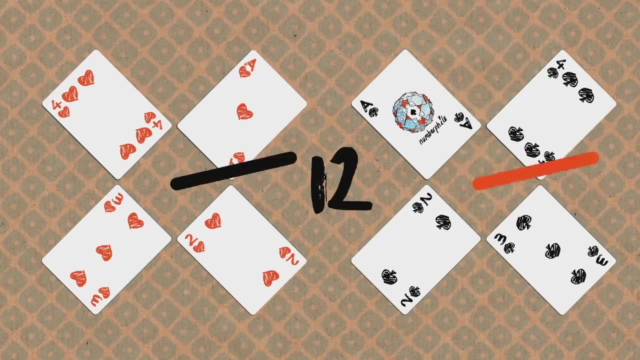 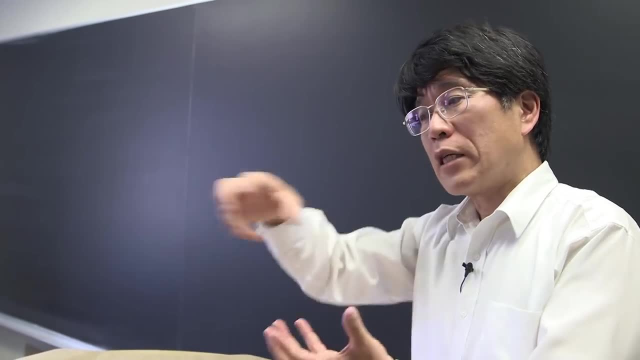 and if you want to go, five, you are here, six here, seven here, eight here, and so forth. you can keep going. Okay, you remember that our way of shuffling was very special. We took the top card and then put it at the bottom. 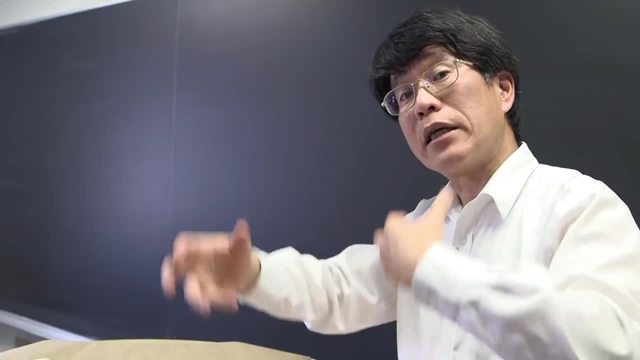 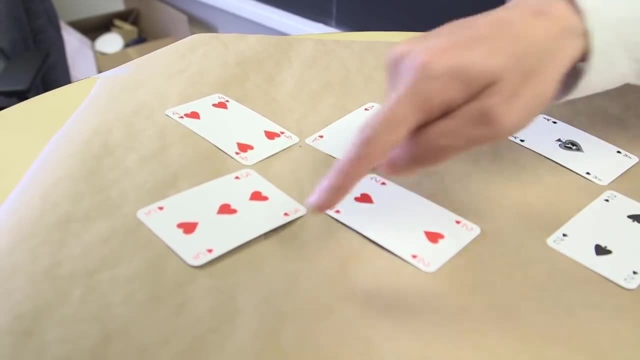 So you, as you keep repeating this, you are cyclically or cyclically depending on the side of the Atlantic- permuting those cards. So you go from here to here, to here to here and keep going, Whereas in the other deck 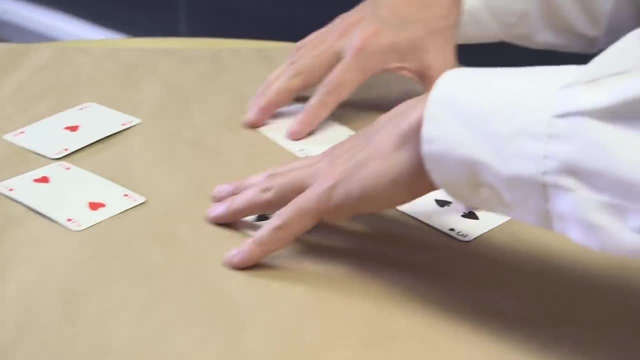 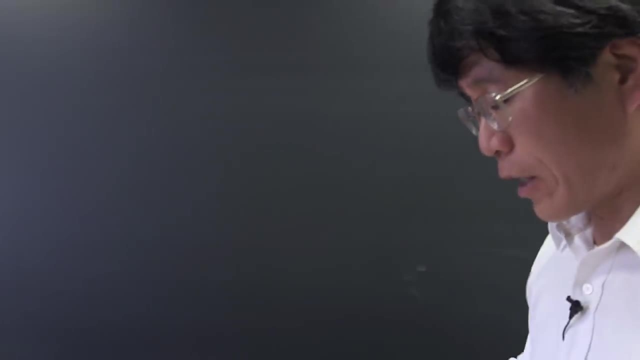 which had the reverse order: you go from here to here to here to here. Okay, we had four cards, but let's generalize and explain a little bit, because this card trick works with any number of cards. in general, Let's say that you have cards one, two, three and so on. 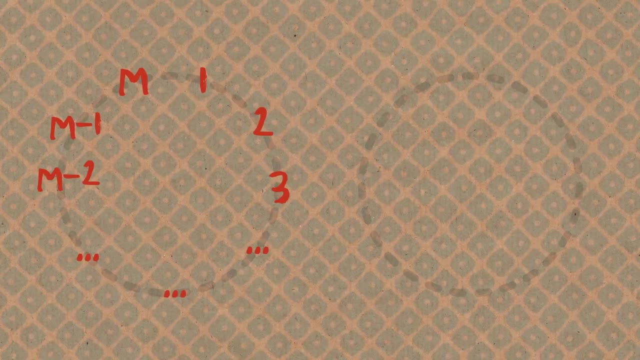 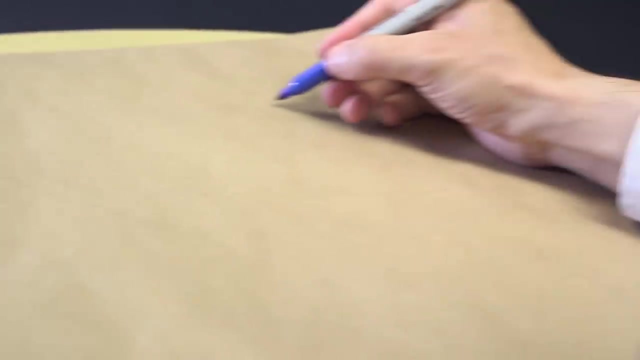 arranged in a cyclical fashion all the way to M. So let's say M minus two. M minus one. M is number, total number of cards, and I choose the letter M for a purpose. On the other side you have the cards in the reverse order. 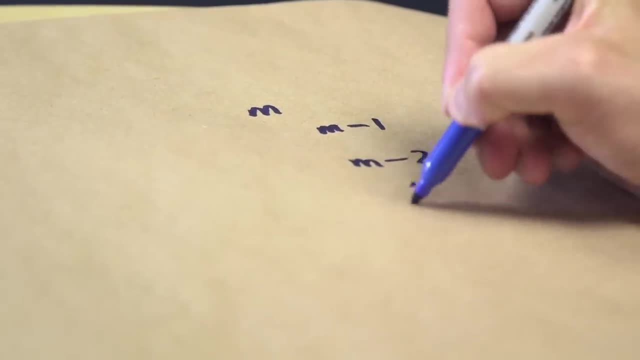 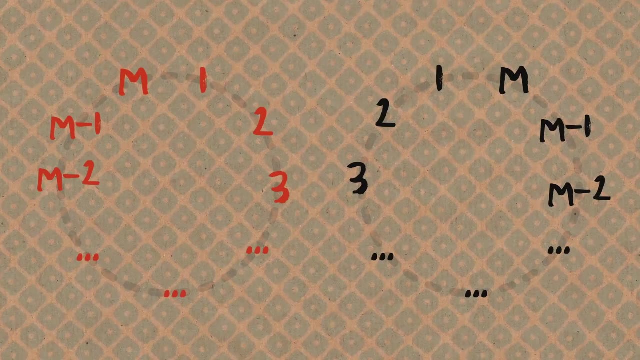 M, M minus one, M minus two, and dot, dot, you keep going, and then three, two, one. you come back like that. okay, So in our card trick M was four, but in general M works. 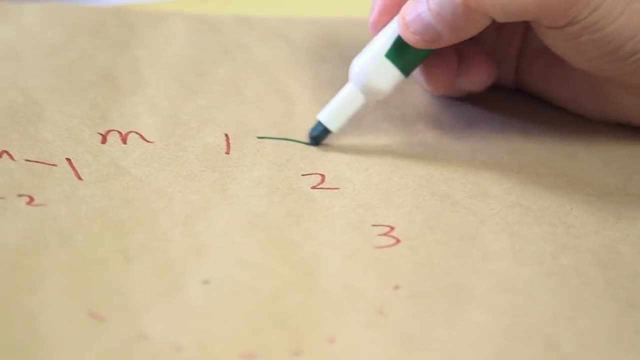 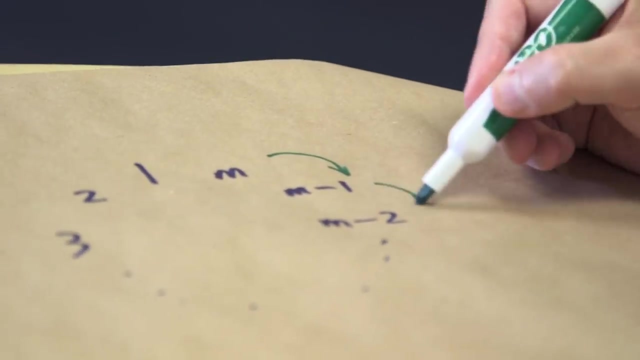 And one shuffle does this: You start from one and it goes to two, and two goes to three, and here you go from M to M minus one, M minus one to M minus two, and that kind of thing. Suppose that on the left that is the red pile. 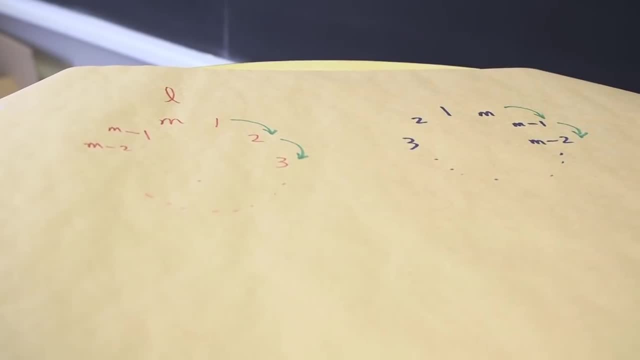 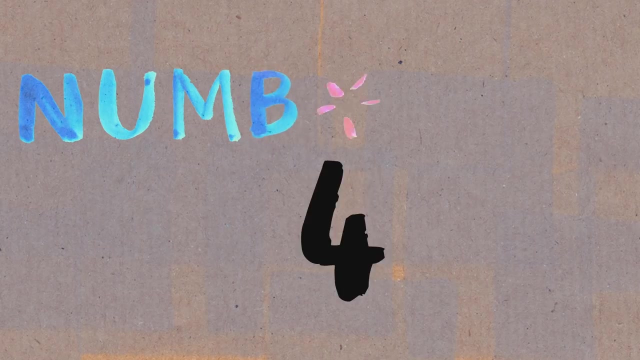 you made L shuffles On the right, you made R shuffles- L as in left, R as in right. Well, the total number of shuffles that we made was the number of letters in number file. N U M B E R. 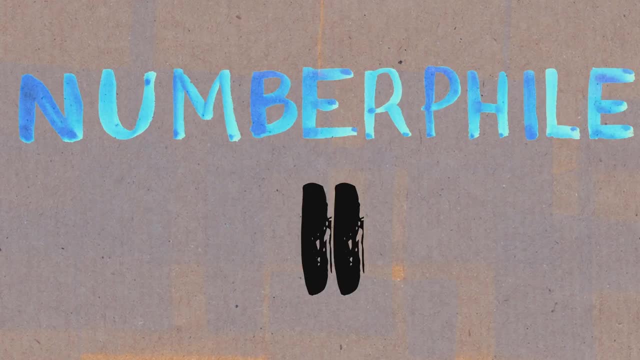 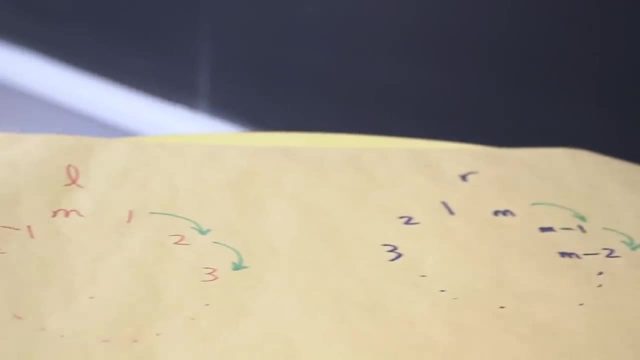 P, H, I, L, E, 11 letters. So we know that L plus R was 11 for us. So L and R are not independent. If you chose to shuffle the red deck L time automatically, you are shuffling. 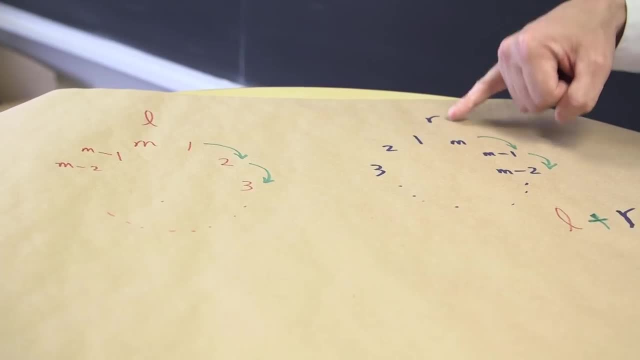 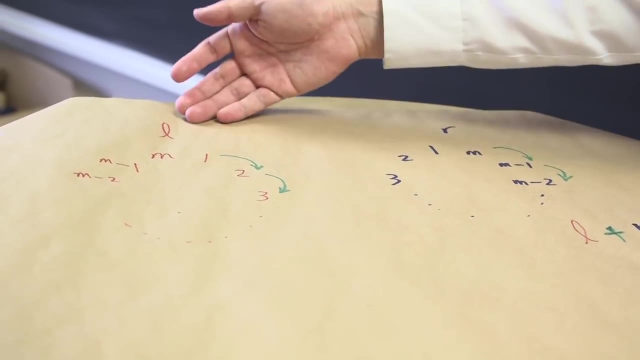 however, whatever else you do, the right deck R times. but R equals 11 minus L And if you choose to shuffle the right deck, that is the black deck R times, you cannot help shuffling the left deck, that is the red deck- 11 minus R times. 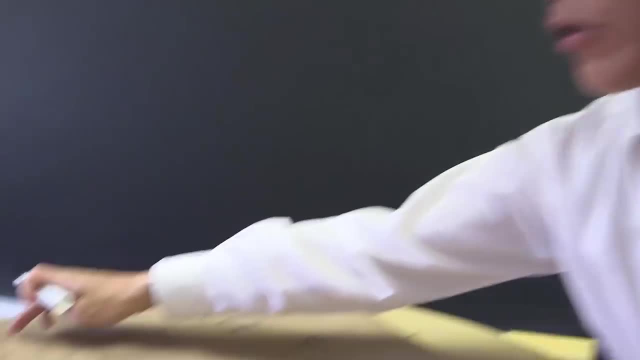 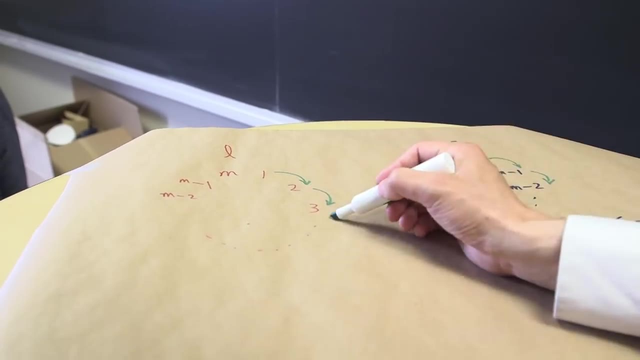 So you have that relationship. So let's start shuffling. Say that you shuffle the red deck L times. One goes to two. so each time you increase by one, two goes three and if you keep going after, L shuffles. 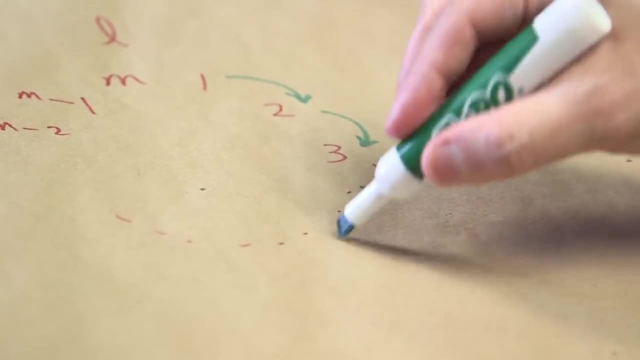 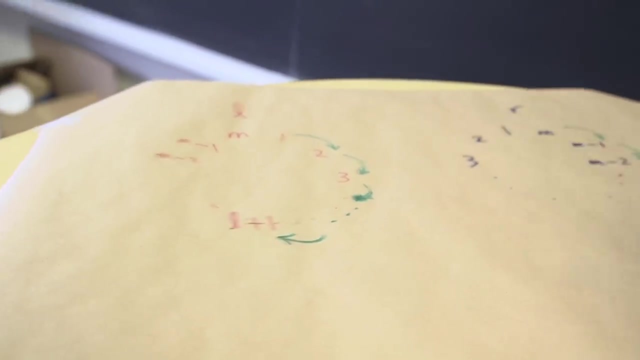 it takes a little bit of thinking to convince ourselves. you arrive at not L but L plus one after L shuffles On the right black deck. after one shuffle you go from M to M minus one to M minus one to M minus two. 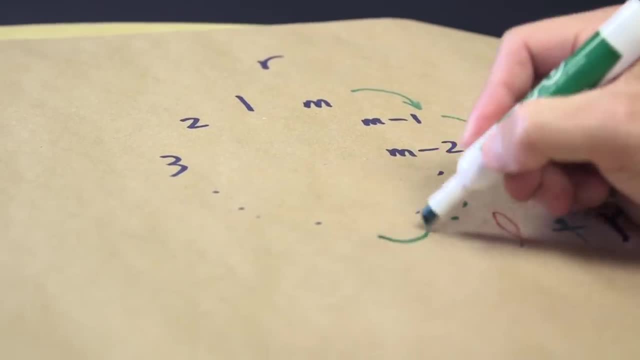 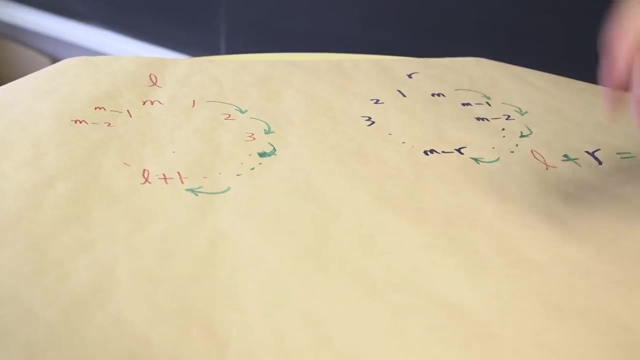 and if you keep going- and that is slightly less confusing- at the end you arrive at, after R shuffles, M minus R. So after those shuffles, the cards that emerge on the top of each deck is L plus one and M minus R. 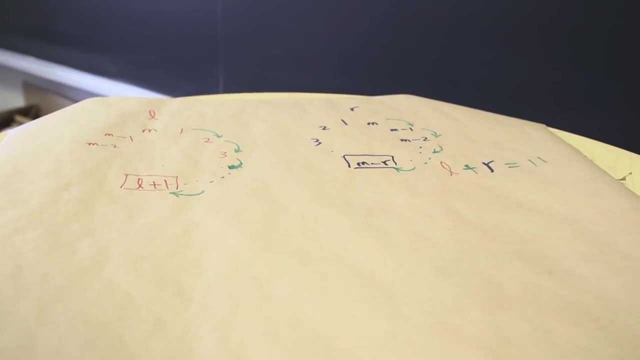 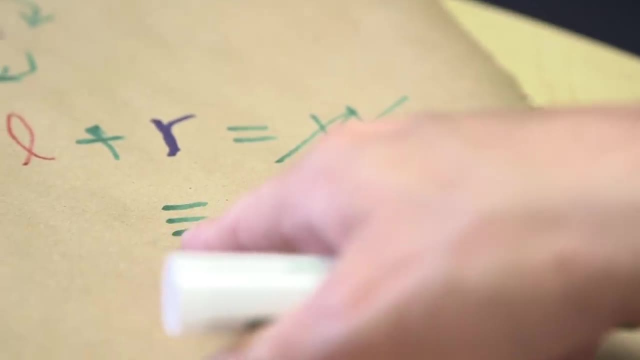 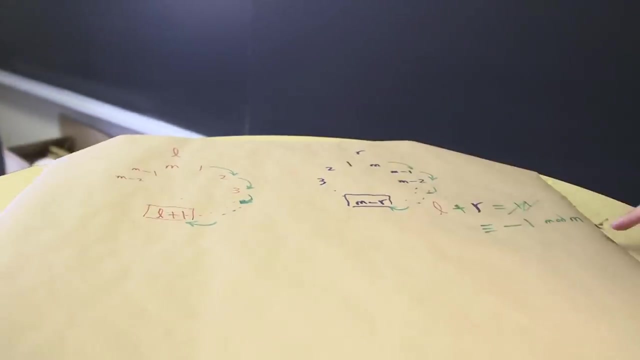 Those two cards emerge, We used 11, but let's say that L plus R was some number more generally which was chosen to be, some number which is congruent to minus one modulo M, where M is the number of cards in each deck. 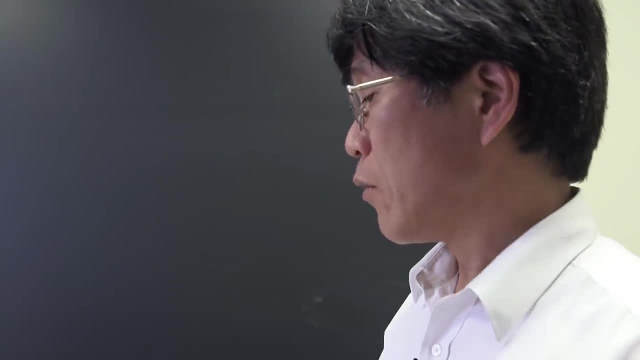 So for us, M was four and for us 11 was the chosen number, and 11 is minus one mod four. by the way, Where have you pulled, yeah, where have you pulled that minus one mod M from? 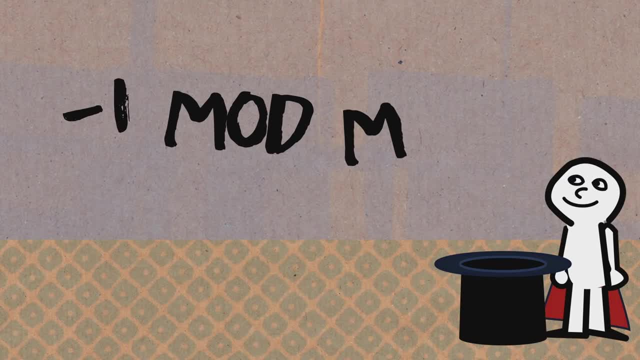 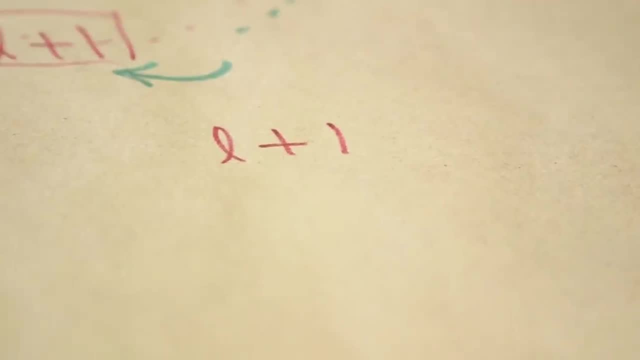 And we'll see why this minus one becomes useful in a moment. That's part of the magic, you see? Okay, all right, all right, You have to do magic at some point, okay? So let's see what L plus one is compared with M minus R. 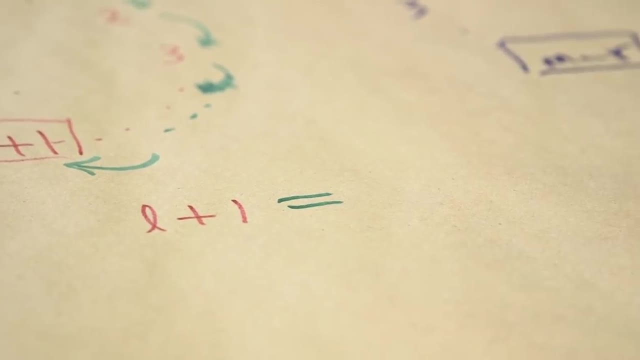 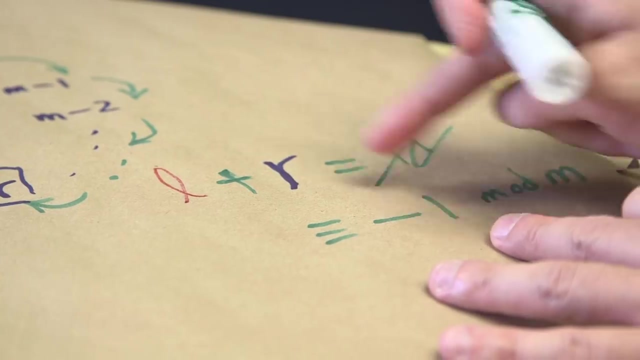 and we'll see that they are actually the same thing, You see, because L, we see, is equal. to look at this, L plus R equals minus one, or congruent minus one. so L equals minus one minus R. 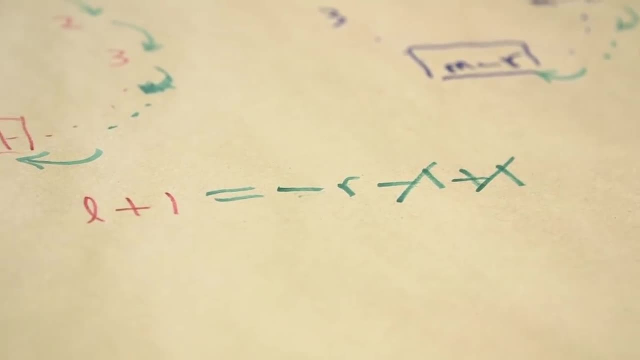 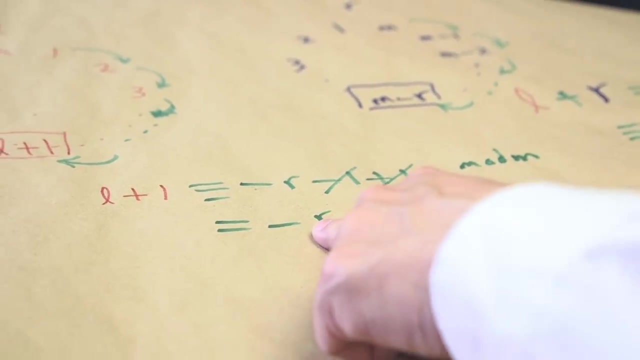 Let's not forget plus one. So minus one and plus one, cancel, and you are left with only minus R. So this is modulo M, But minus R can be written by modulo arithmetic again as M minus R. that's the same thing: modulo M. 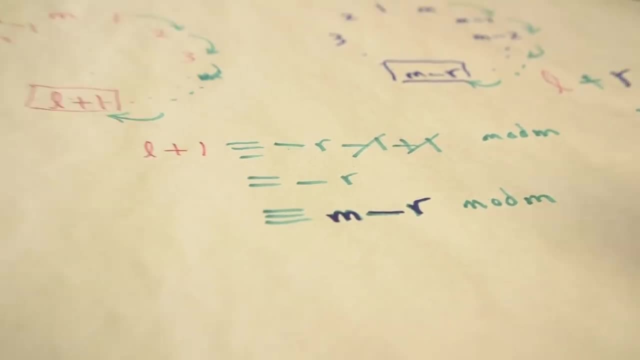 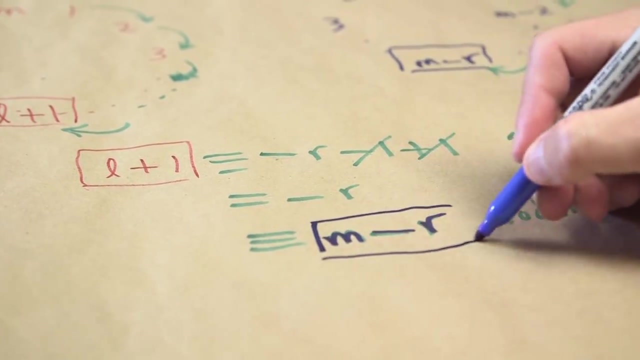 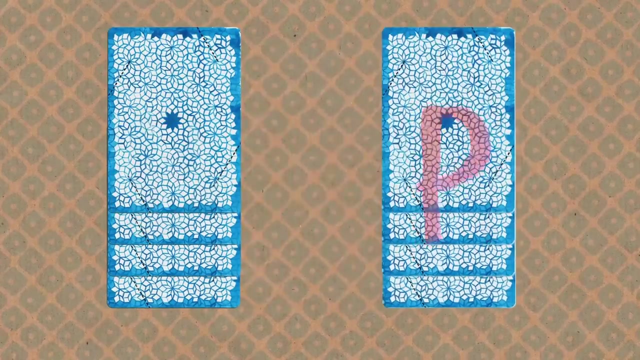 Drawing it like that. okay, And so what we see is that modulo M, L plus one the top of the red deck and M minus R top of the black deck, They are actually the same. So after those shuffles, the same cars emerge on the top. 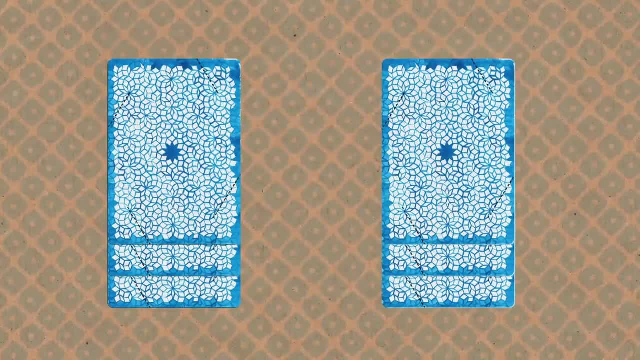 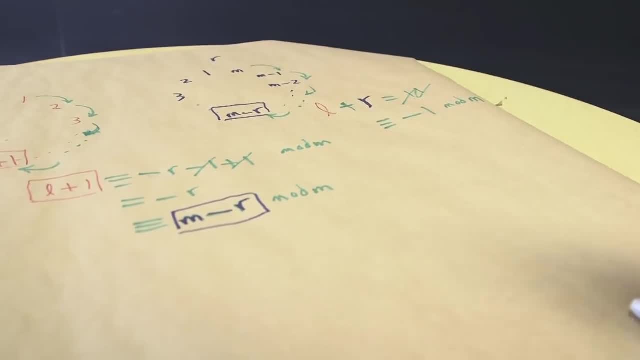 You put them aside. now you have to start over again, and then the number of cars M changes. But that's where minus one becomes useful. 11, that we chose- that's number of letters in number file- has the beautiful property that it is indeed congruent. 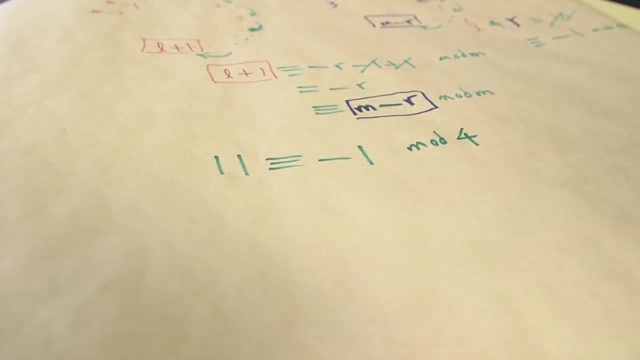 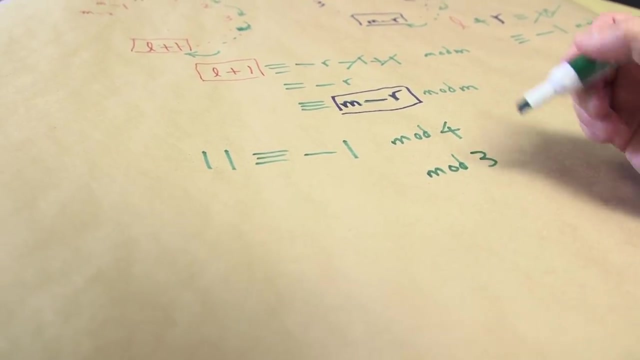 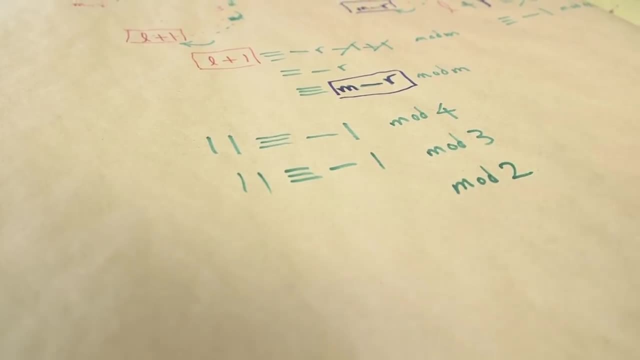 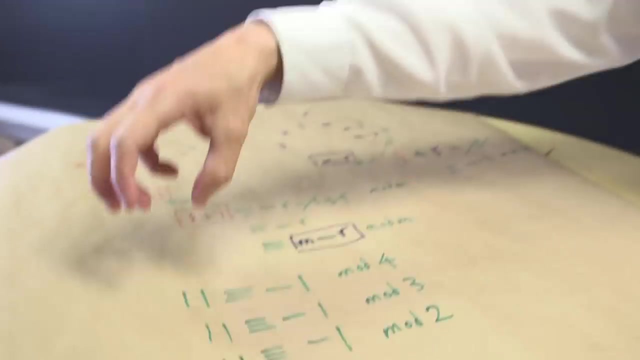 And next stage: you have lost one pair of cars. you have to do mod two, but amazingly, 11 is also minus one mod two, And that is why this number, magic number, key number 11, worked, just as you descended. 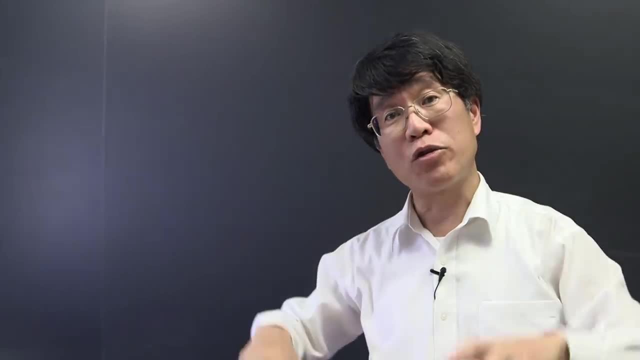 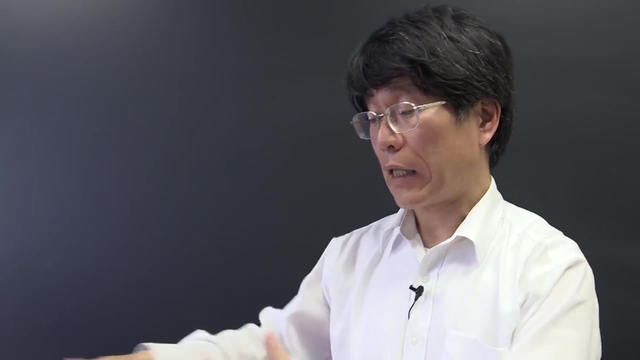 those different moduli, the chain where they are: mod four, mod three, mod two, And that's how I chose 11.. Or if you want to do this car trick with other parameters, for example with larger number of cars and 10, and 12,. 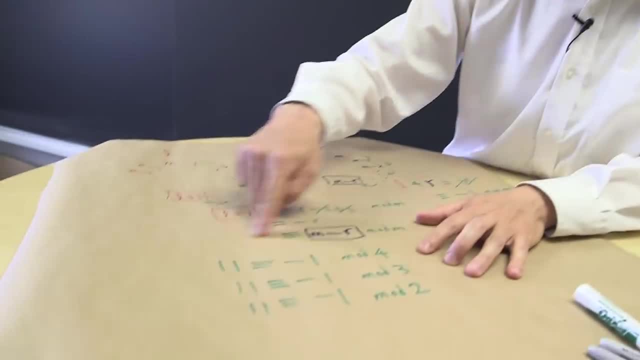 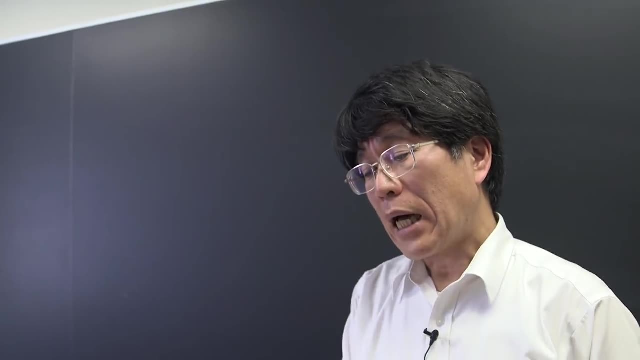 and so forth and so forth. all you have to do is to solve this, what is called simultaneous system of congruences, Like simultaneous system of equations, but you are doing modular arithmetic And there is a way of doing this, called Chinese remainder theorem. 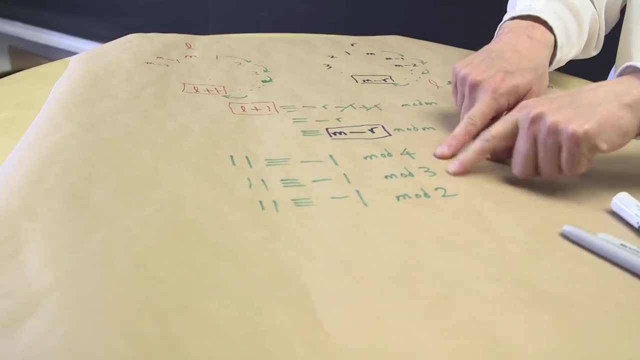 By the way, the standard way we teach and learn Chinese remainder theorem has modulated a co-prime. They should all be modulated, They should all be co-prime. But this is a tricky case of Chinese remainder theorem because, for example, two and four are not co-prime. 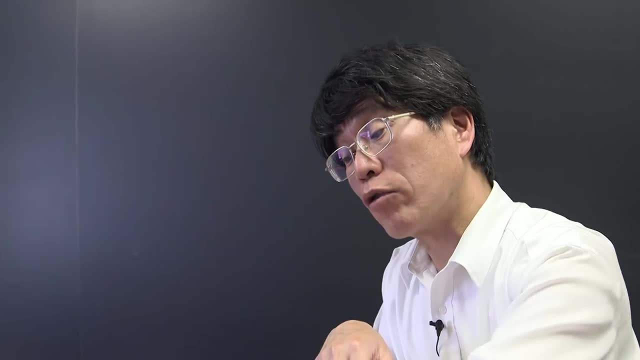 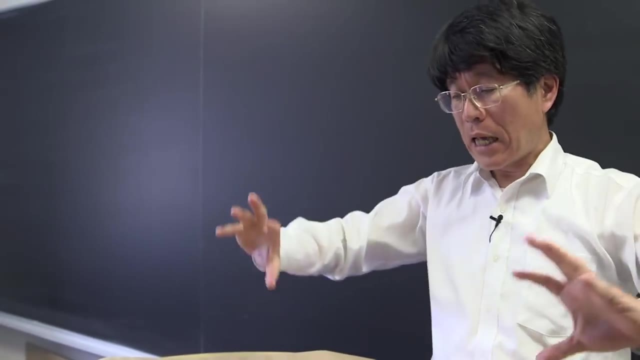 But even there there is a version of Chinese remainder theorem that works. So this kind of congruence system, congruence is always solvable. So you give me any m, So use a lot of cards if you like. 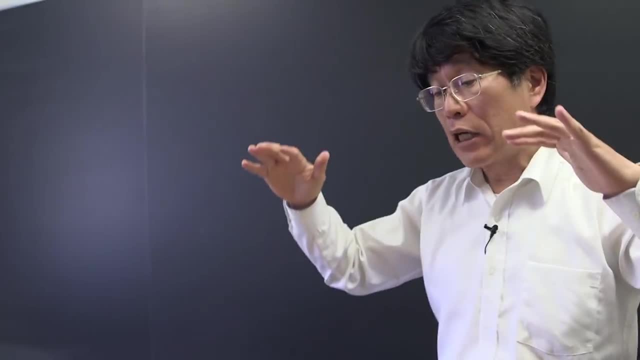 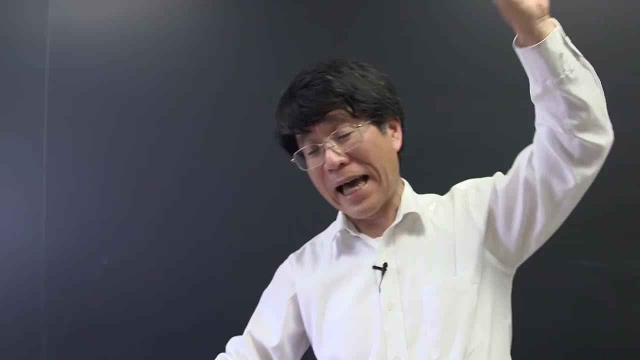 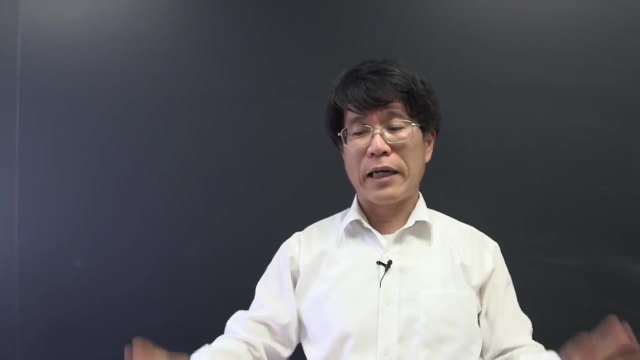 But just reverse the orders here and here And you find some key number which is equivalent to 11, but some x which is minus one mod m. Also minus one mod m minus one. Minus one mod m minus one. So all the way down all those moduli. 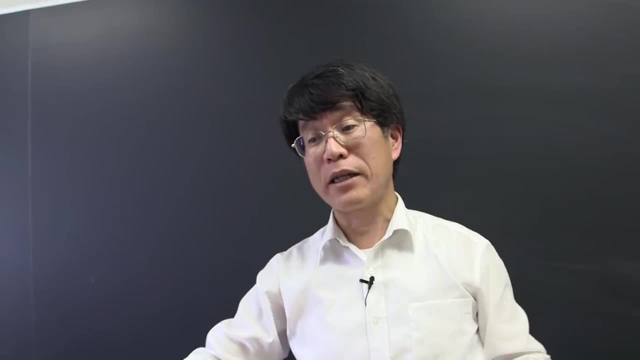 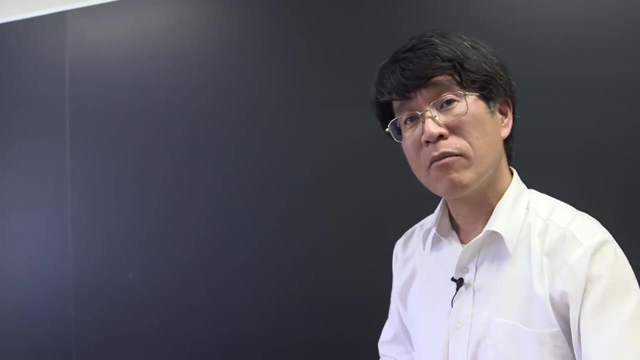 you should always be minus one. You should solve those simultaneous equations for x And using that number of phrases. this trick always works. So if I had two piles of 10, there'd be some other word I'd be having to use. 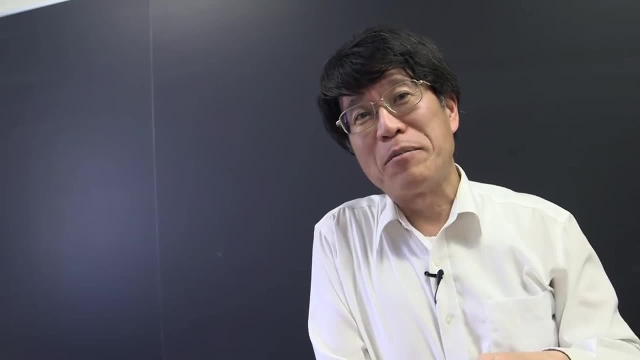 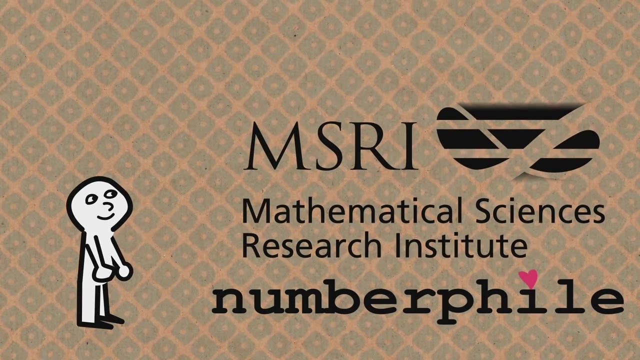 That's right, But it would be a longer phrase and longer word. But I'm sure it would be some word like a number file which would be of special significance to you If you'd like to try your hand at some of the mathematical problems that we've talked about. 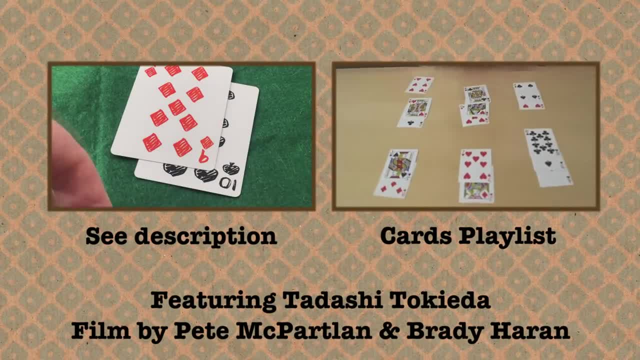 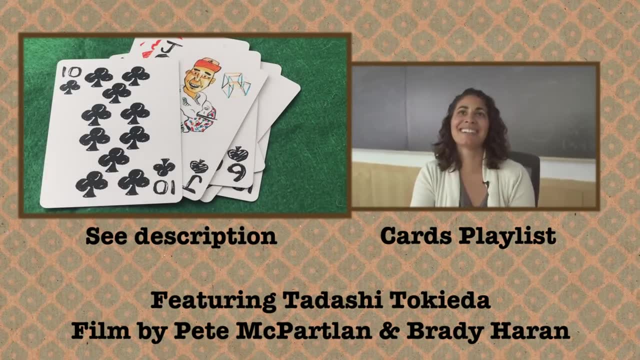 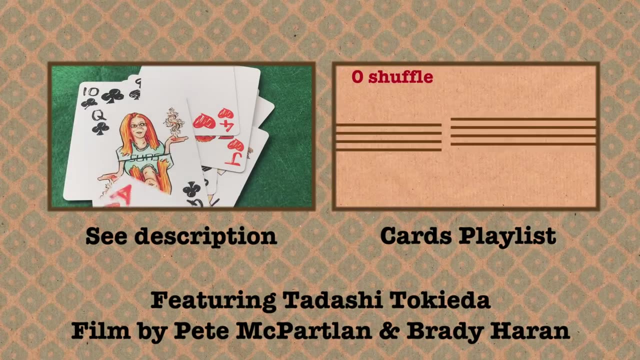 the mathematical card tricks you've seen on Numberphile, but don't own a deck of cards, well, you could try these Numberphile ones. There's a link with more information about them down in the video description, And if you'd like to see more videos about playing cards, well,